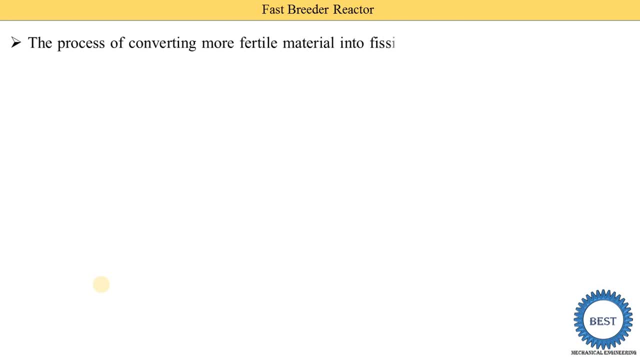 So now, what is the meaning of the breeders? Breeder means the process of converting more fertile materials into fissile materials in a reactor is known as a breeding process. So we understand the two things: No moderator is used and in this reactor, fertile material. 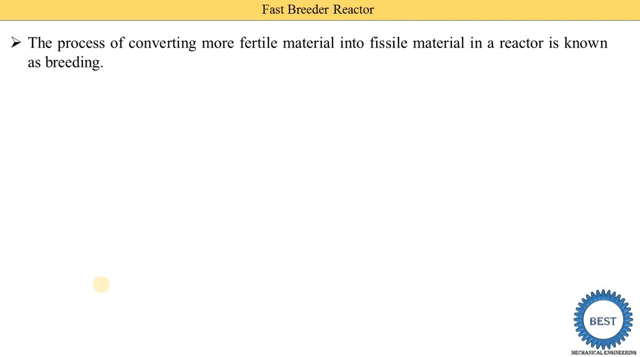 is converted into the fissile material. It is called as the breedings. So it is important. lies in consequence that all the available fertile materials can be converted into fissile materials. Fissile material means they are able to convert the fertile materials into fissile materials. So it is important. lies in consequence. 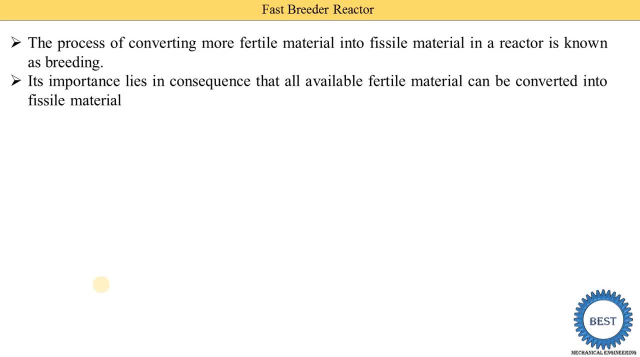 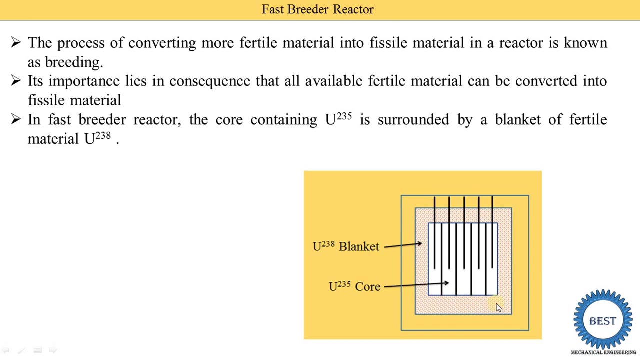 carried out fission reaction. It is called as the fissile materials. So in a fast breeder reactor, the core containing uranium-235 is surrounded by blanket of fertile materials, uranium-238.. So here you see. this is the. uranium-235 is used as a fuel or a core. So 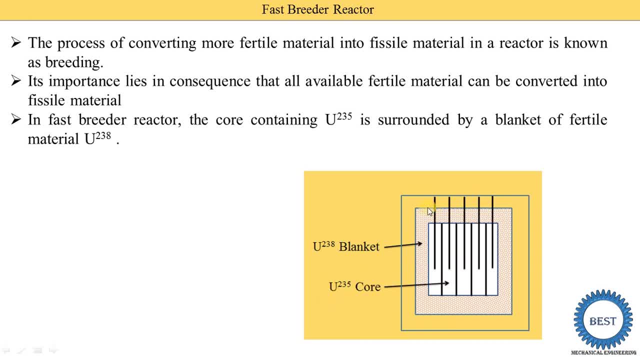 uranium-235 is the core and instance of this moderator. this core is surrounded by using this uranium-238 means it is called as the blanket of uranium-238. So when this fission reactions of this uranium-235 is started, at that time this uranium-238 is absorbed. 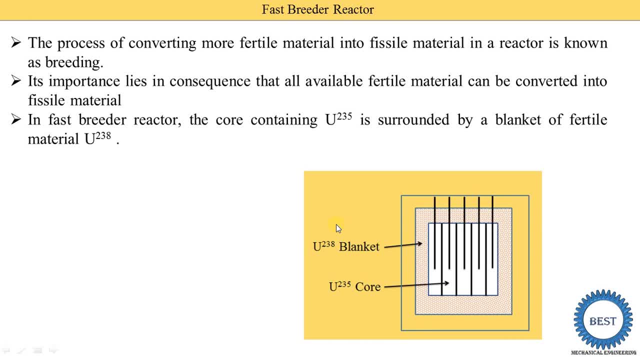 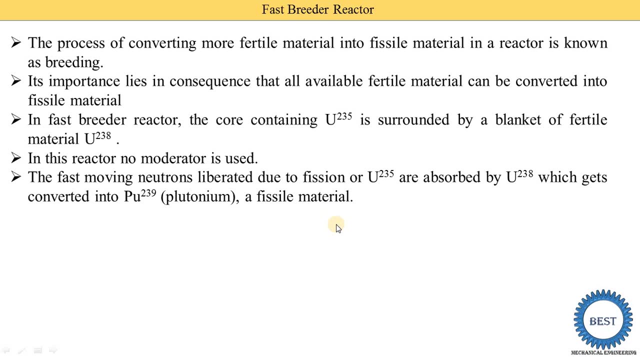 some neutrons and this material is converted into fissile materials. So in this reactor no moderator is used. The fast moving neutron liberated due to the fission Of uranium-235 are absorbed by uranium-238.. So when we carry out the fission reactions, 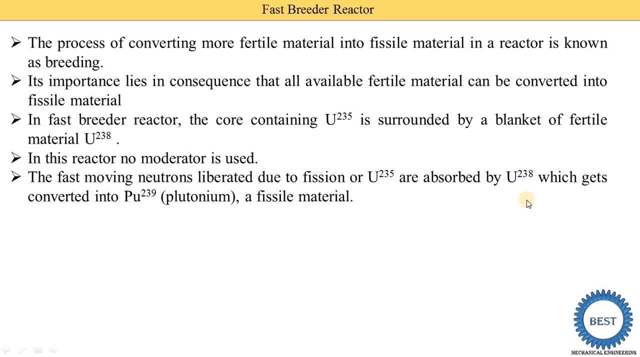 of the uranium-235, at that time these neutrons are liberated and these neutrons are absorbed by uranium-238 and which gets converted into plutonium-238 as a fissile materials. It means uranium-238 is converted into Pu-230.. 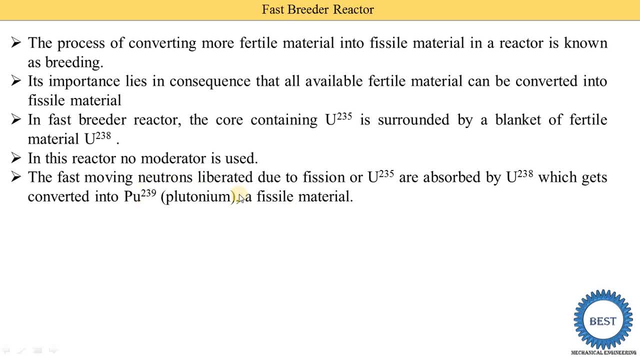 And the Pu-239 is the fissile materials and this material is again using some nuclear power plant to carry out the fission reactions. These manmade fuel, Pu-239, can be used for further fission reactions and similarly, thorium Th-232 can be converted into uranium-233 means instance of uranium-238, we are able to also. 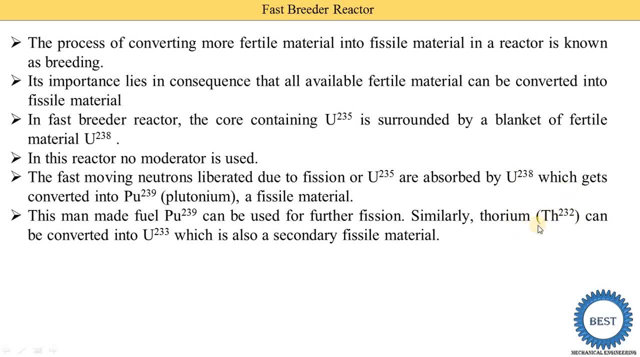 use the thorium-238. So we can use the thorium-232, and this thorium-232 is converted into uranium-233 means as a blanket, we can use uranium-238 or a thorium-232.. Therefore, these types of the reactor are important, since they not only produce the 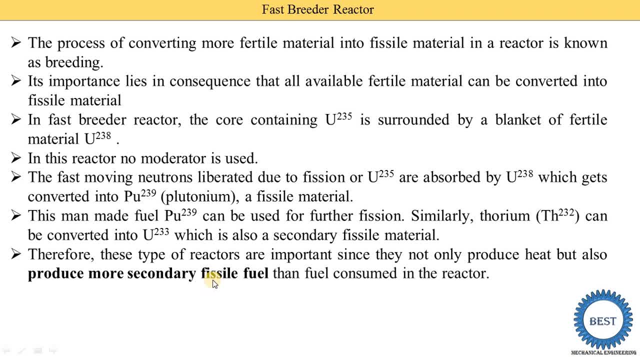 heat but also produce the more secondary fissile materials than the fuel consumed in the reactors. Means fast breeder reactor are fulfilled the two purpose: One is to produce the heat energy. The steam is produced and it is supplied to the turbine and the turbine is produced. 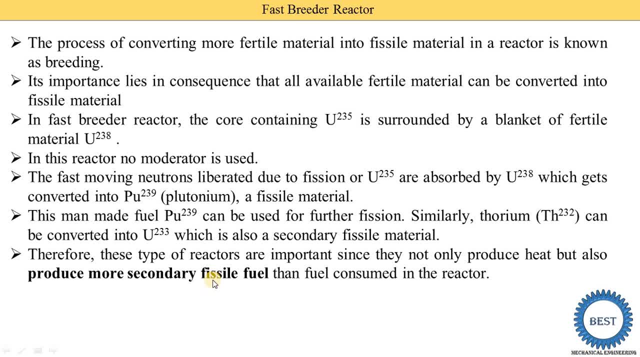 this mechanical energy. And second function: they are produced the fissile fuels. they are used in some other nuclear power plants. India has massive reserve of thorium, means the in India the large quantity of thorium is available and limited reserve of uranium are available. 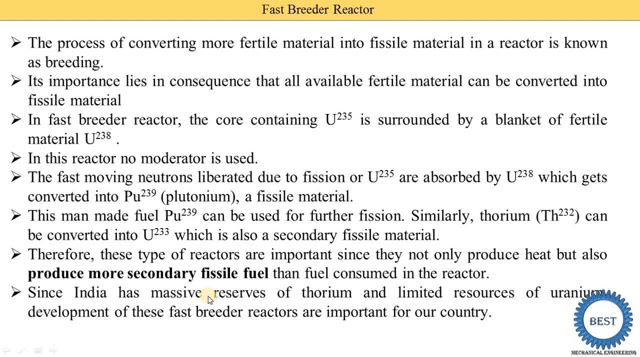 Okay, So development of these fast breeder reactors are important for the production of thorium. Okay, So in a fast breeder reactor we convert these thoriums into uranium-233.. So if you develop a fast breeder reactor, in a fast breeder reactor we convert these. 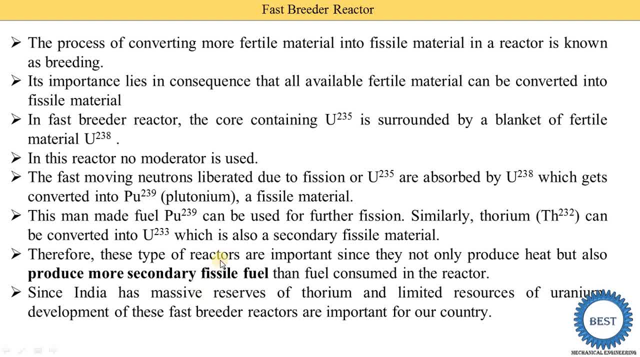 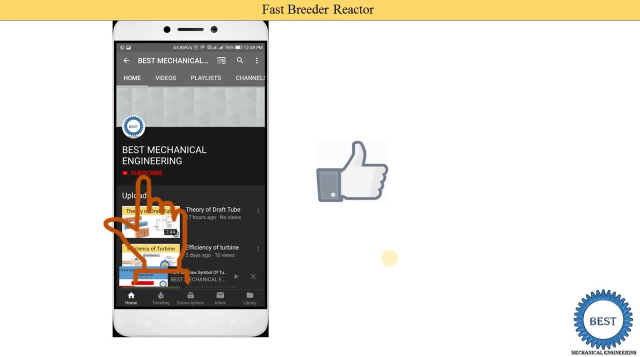 thoriums into uranium-233.. And uranium-233 is the fissile material, So it is a benefit for the our country. Now, before moving out, I request to like the video and subscribe my channel for watching the more videos related to power plant engineering or other subject of this mechanical engineering. 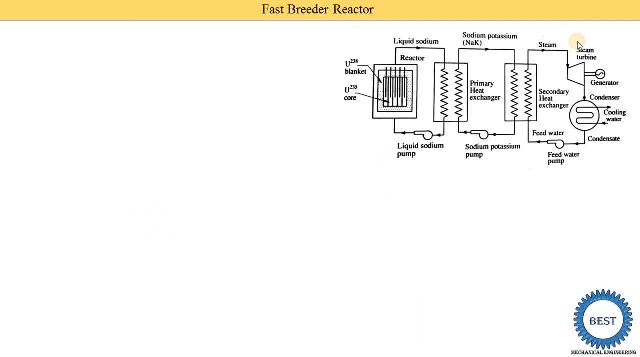 For power plant engineering. the link is provided in the description as well as in the card for other subject. Thank you all. If you like this video, please subscribe to our channel For more videos related to the Power Plant Engineering or other subject of this mechanical engineering. 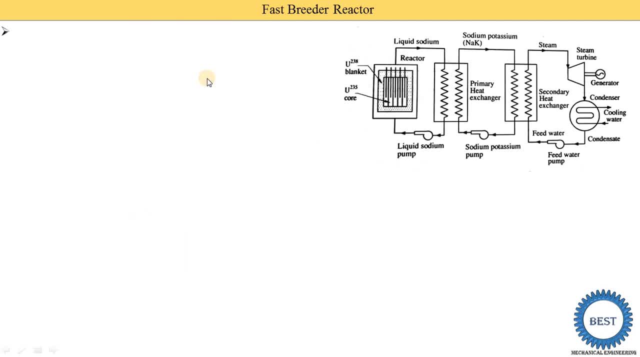 for other subject. i request to visit playlist. now, here you see, this is the arrangement of liquid metal- fast breeder reactor. liquid metal, fast breeder reactor means in our heading we can add this: liquid metals means this liquid metal is used as a coolant. okay, and as a liquid metal. 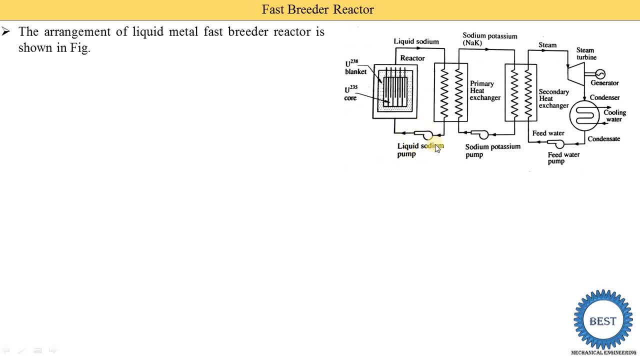 we use the liquid sodium, okay. so here you see, this is the liquid sodium pump is there? so this liquid sodium is supplied in these reactors and this liquid sodium is absorbed, this heat energy. okay, and they are supplied in primary heat exchangers, okay, so now we understand in this. 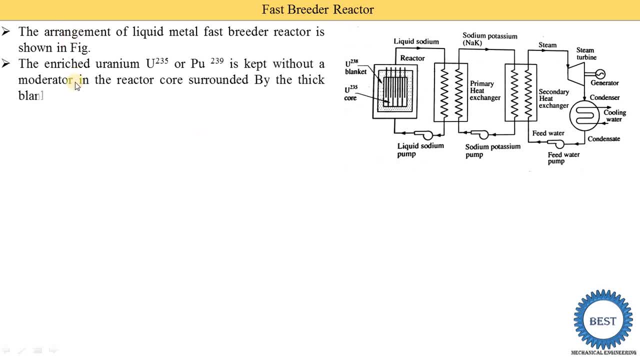 detail: the enriched uranium 235, or pu 239, is kept without a moderator in the reactor and this core is surrounded by the thin blanket of depleted uranium 238. okay, so as a reactor, we use the uranium 235 and the blanket of uranium 238 is used, and this coolant is liquid sodiums. 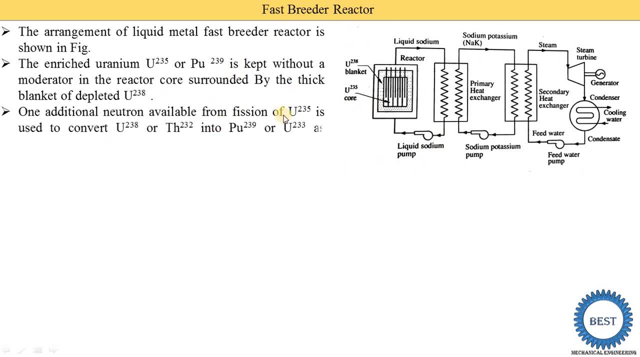 one additional newton available from fission of uranium 235 means here we use the fuel that is uranium 235. okay, so when this fission reaction of the uranium 235 is carried out, at that time the newton is liberated and this newton is supplied to this blanket, and as a blanket we 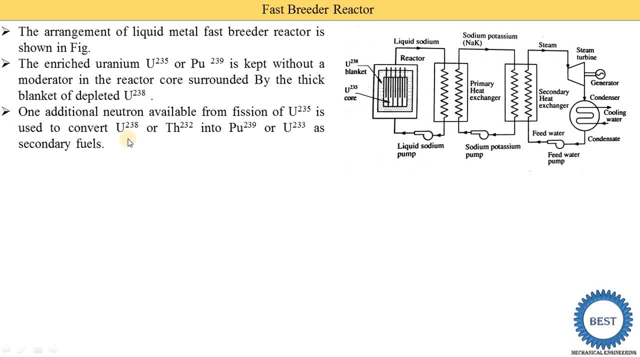 are able to use the two fuels. one is the uranium 238 that we you see here. okay, so when this uranium 238 absorb the newton, it is converted into pu 239. if we use the blanket of thorium 232, then it is converted into uranium 233. 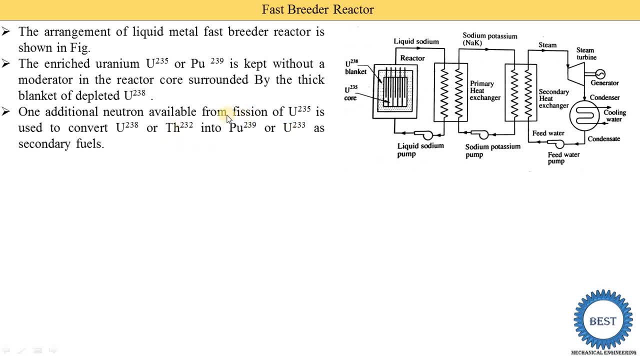 okay, and this thorium- sorry, this pu 239 or a uranium 233 is further used as a secondary fuels in some other reactors. so these reactors also use two liquid metal coolant, in which sodium is used as a primary coolant and sodium potassium is used as a secondary coolant. okay, so here you see. this is the primary heat. 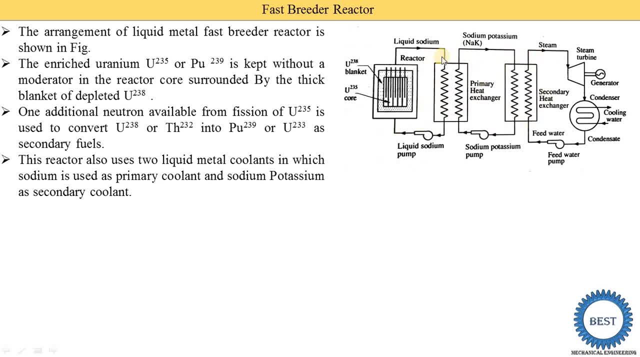 exchanger. this is the secondary heat exchangers. okay, so this is called primary circuit, this is called the secondary circuits and this is the final circuits. okay, so in this primary circuit the coolant is used, that is, the liquid sodiums. in the secondary circuit, that is a sodium potential. 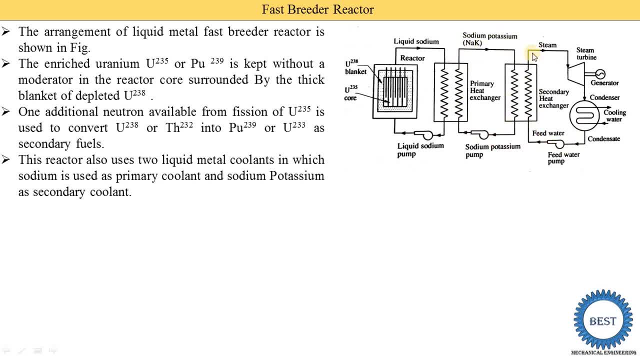 is used and in the third circuit the water is enters and it is converted into the steam means. in a third circuit the working substance is a steam. liquid sodium is circulated through a reactor to carry the heat produce. so this liquid sodium is supplied in this reactor. they absorb the heat. 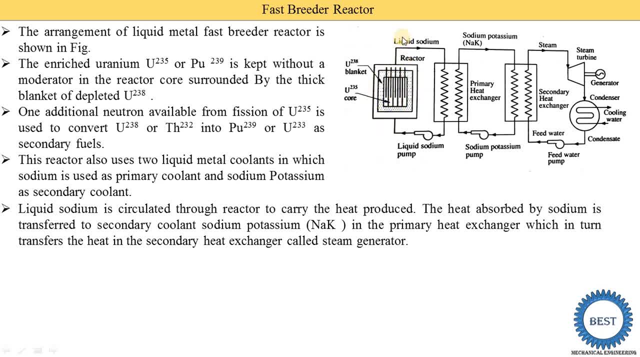 energy and its temperature is increased and then it is transfer to this primary heat exchangers. okay, so in this primary heat exchanger, this liquid sodium is supplied heat energy to the sodium potentium. okay, and sodium potentium is supply its heat energy to the secondary heat. 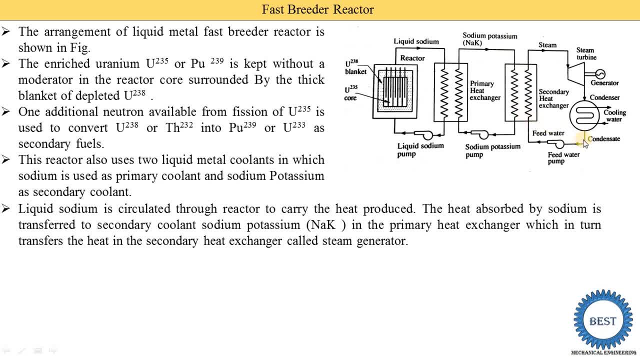 exchangers. in this secondary heat exchangers, the feed water coming out from this pump is heated by using this sodium potentium. okay, and this steam is produced. this steam is supplied in a steam turbine. in a steam turbine, this mechanical energy is produced. mechanical energy is produced. 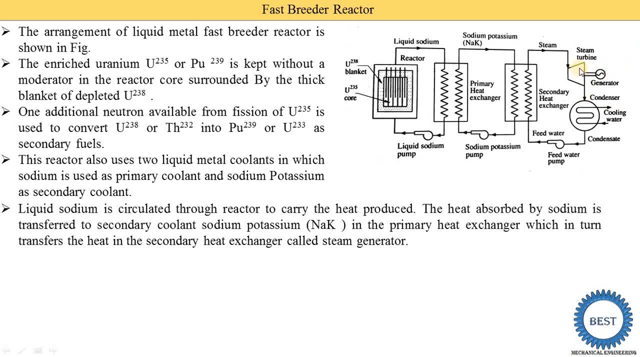 is supplied to the generators and, finally, electric city is produced. steam coming out from the turbine is supplied in condenser. in a condenser, steam is converted into the water. this water is supplied in feed water pump and this water is again supplied to this secondary heat exchanger. 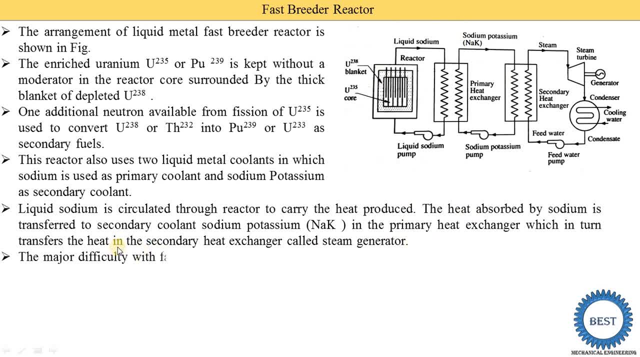 this way, the cycle is continuously run. the major difficulty with fast breeder reactor is to remove the large quantity of heat from the core, as the power density is very high, which is 40 times greater than the cando type reactors, 30 times greater than the bwr means boiling water reactors. 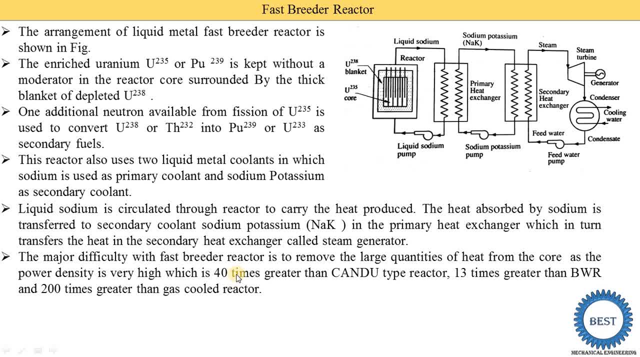 and the 200 times greater than the gas cooled reactor means its power density are very high compared to all other types of these nuclear reactors. therefore, special coolant and the special arrangement of liquid jet, whose gas is produced through the corne air or the gas cooled, are necessary to carry out the large quantity of heat from the reactors. now we understand the 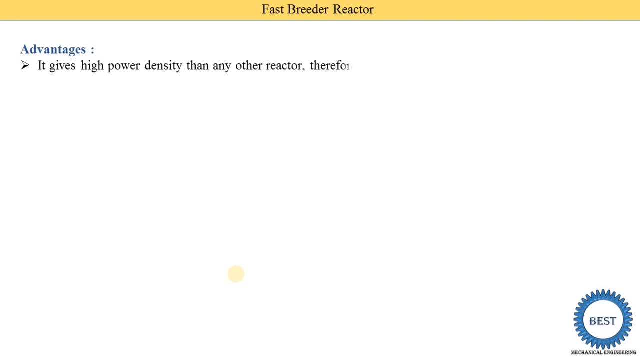 advantages. first advantage: it gives high power density than other reactors. okay, so already we see the digit 40 times 100 times 10. okay, therefore the small core is sufficient. second: moderator is not required. third secondary: fissile materials by breeding are of ten, means we are, you produce.